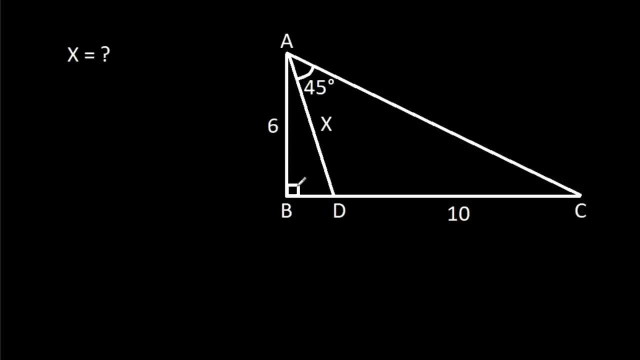 In this video we have been given a right angular angle in which AB is 6,, CD is 10, angle CAD is 45 degree and AD is X, Then we have to find X. So the first method: if we extend AD to suppose E and if we join CE such that this angle is 90 degrees. So the first method, if we extend AD to suppose E and if we join CE such that this angle is 90 degrees. So the first method, if we extend AD to suppose E and if we join CE such that this angle is 90 degrees. 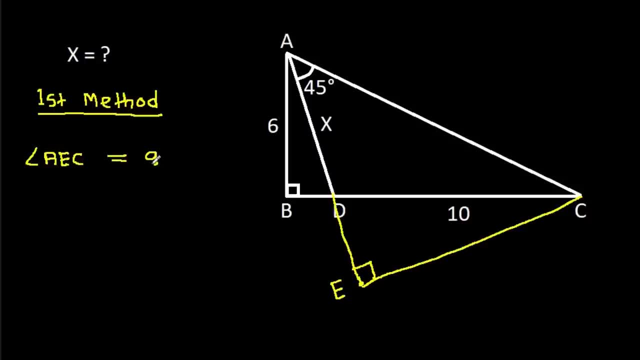 Angle AEC. it is 90 degree. It is our construction. And now inter angle AEC. This is AEC. This angle is 90 degrees, This angle is 45 degrees. So this angle, it will be 180 degrees minus 90 degrees, minus 45 degrees. 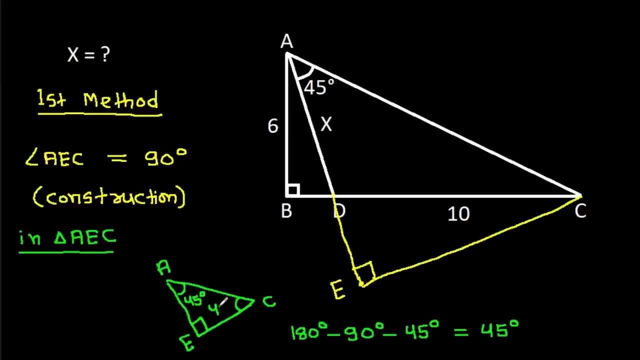 That will be 45 degrees. So it is 45 degrees And now we have angle ZX880.. angle EAC is equal to angle ECA. That means EA, it will be equal to EC. And suppose DE is Y, then EA it will be X plus Y, So EC it will be also X plus Y. 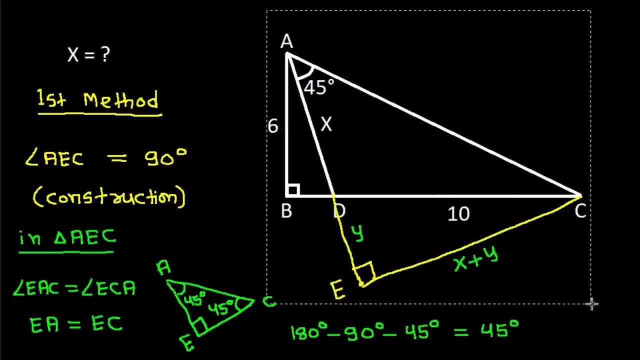 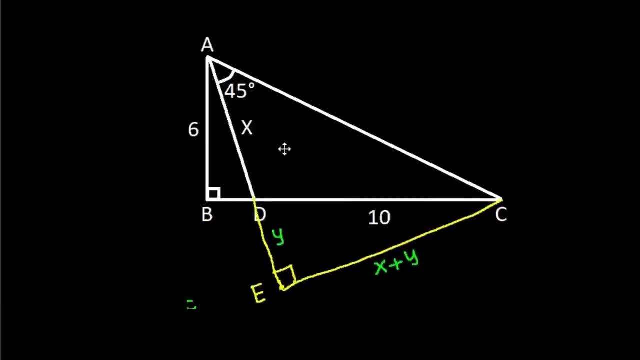 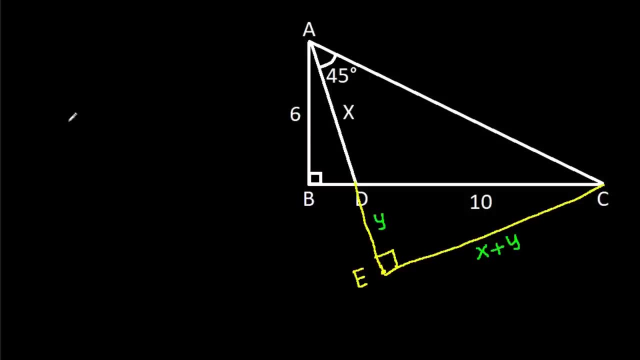 And now in triangle ABD and triangle CED we have: angle ABD is equal to angle CED, that is 90 degree, And angle ADB it will be equal to angle CDE. that are opposite angles, These two angles. 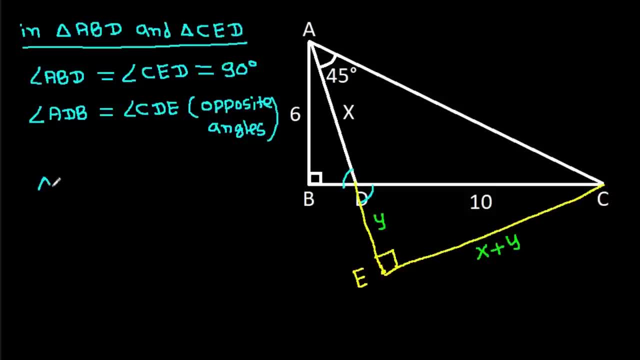 they will be equal. So triangle ABD it will be similar to triangle CE. that is 90 degree. Now angle WH isハ. this angle Batman become ha B by cE, so it is angle ABD, Hence AB by CE it will be equal to ABD. by ED it will be equal to AD by CD And AB6 by CE is. 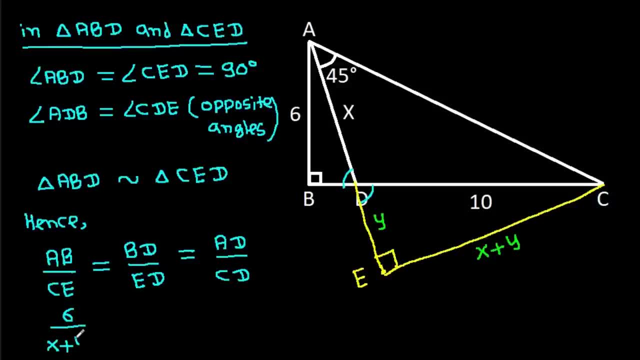 Ax plus H. this can also be equal to AD plus X by CD, which is equal to AB3. by X- y, it is equal to BD. here inter angle, ABD, AD is x, AB is 6 and this angle is 90 degree. 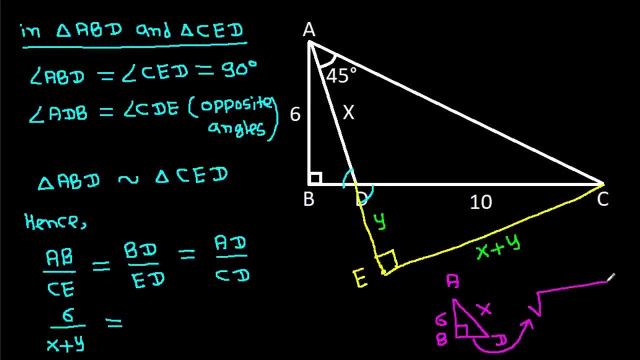 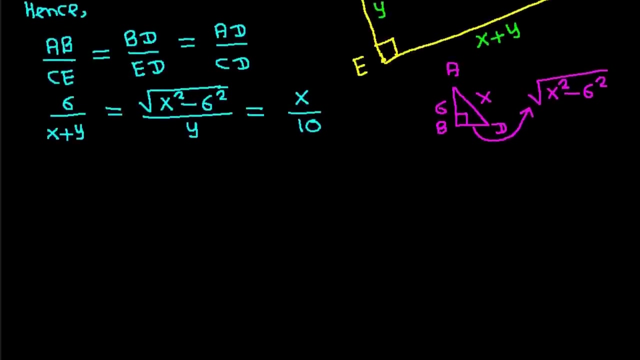 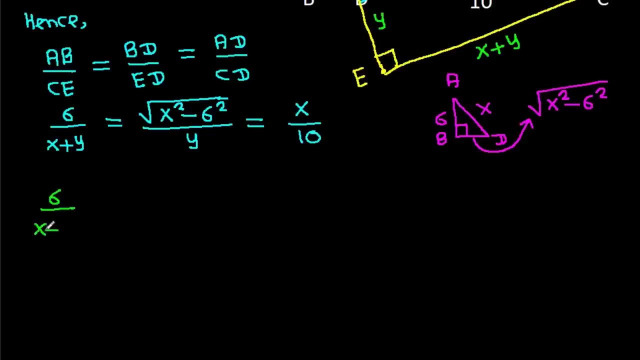 So BD, it will be a square root of x square minus 6 square by Pythagoras theorem, So BD, it is a square root of x square minus 6. square by ED is y, it is equal to AD, it is x by cd is 10, and now we have 6 by x plus y is equal to x by 10. and if we cross multiply. 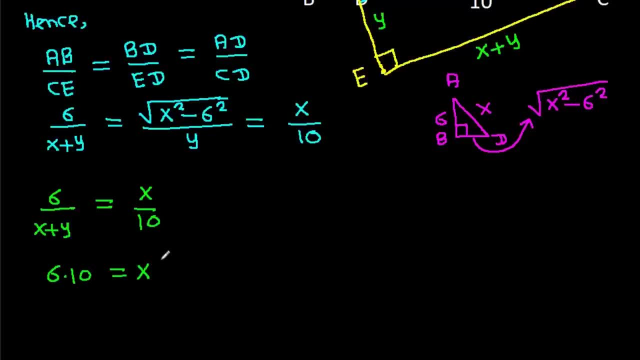 then 6 times 10 it will be x times x plus y and 60 it is x square plus x- y. and also we have a square root of x square minus 6. square by y is equal to x by 10. and if we cross multiply, then 10 times a square root of x square minus 6 square it will be xy. 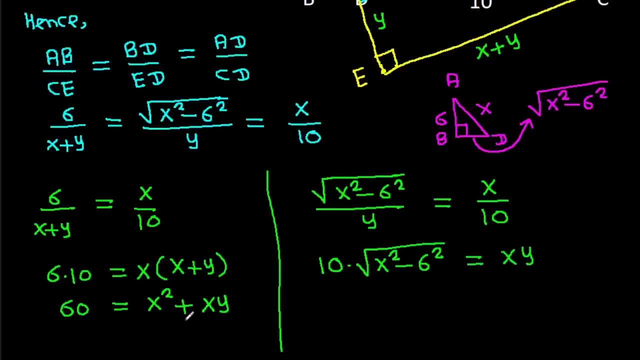 and from here we can get: xy is 60 minus x square, so 10 times a square root of x square minus 6. square by y is equal to x by 10 and if we cross multiply, then 10 times a square root of x square. 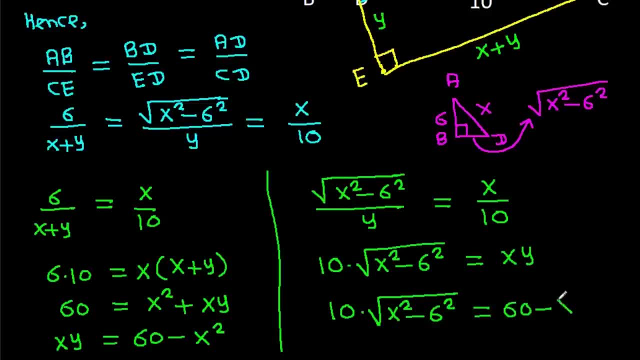 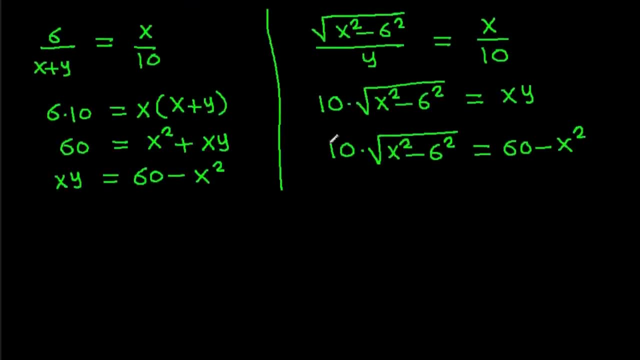 it is equal to 60 minus x square and if we square it both side then it will be 100 times x square minus 6 square is equal to 60 square plus x square minus 2 times 60 times x square and it is 100 x square minus 36 times 100. 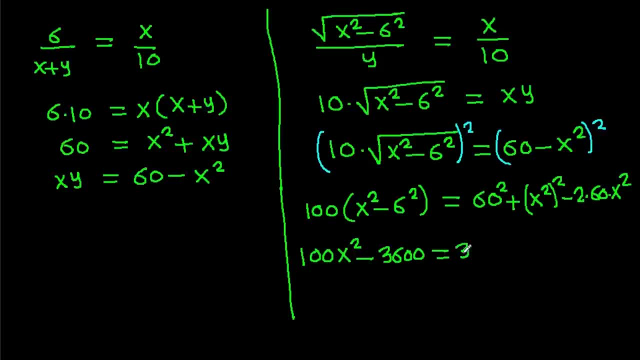 will be 3600, it is equal to 3600 plus x power 4 minus 120 x square, and it is x power 4 and minus 120 x square, minus 100 x square, it will be minus 220 x square, and 3600 plus 3600 it will be 7200, it is equal to 0.. 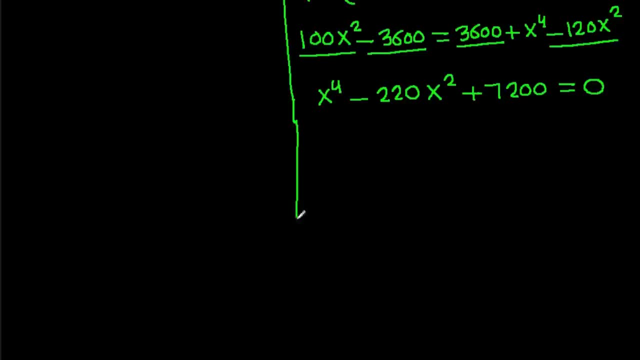 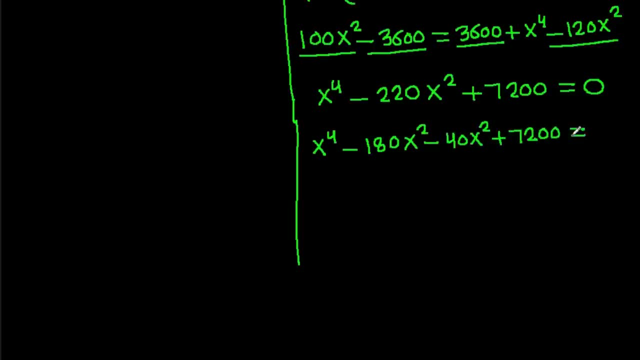 and it is x power 4 and minus 220 x square, it is minus 180 x square minus 40 x square, and it is x power 4 and minus 220 x square, it is minus 180 x square, minus 40 x square. plus 7200 it is 0. and here we can take x square common and it will be x square minus 180. 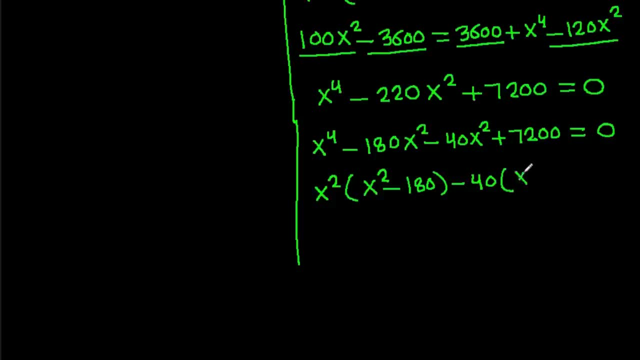 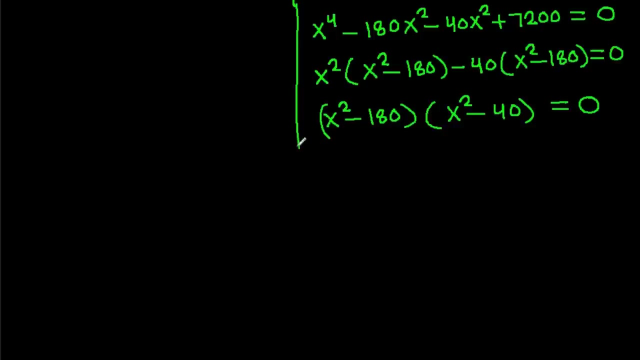 and here we can take minus 40 common, and it will be x square minus 180, that is 0. and now we can take x square minus 180 common, and it will be x square minus 40, that is zero. so either x square minus 180, it can be 0, so x square. 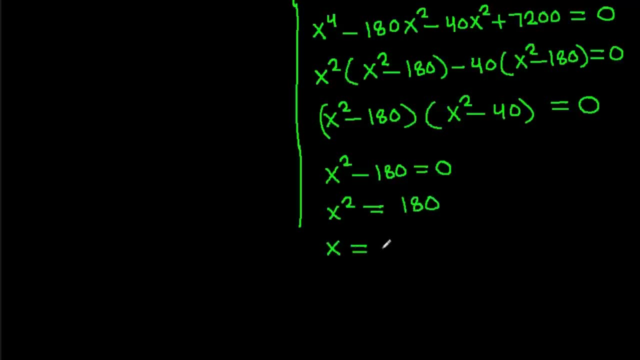 it will be 180 and x will be a square root of 180. so we get: x is 6 times a square root of 5. And either x square minus 40, it can be 0. So x square it is. 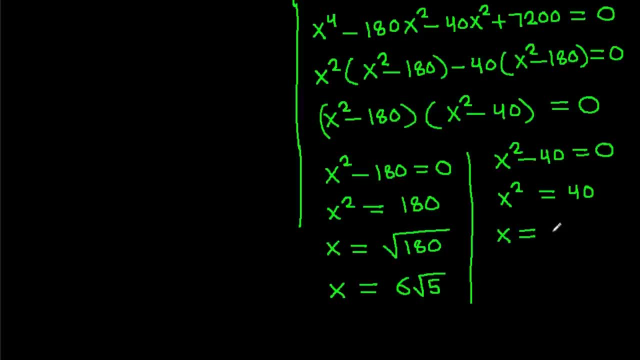 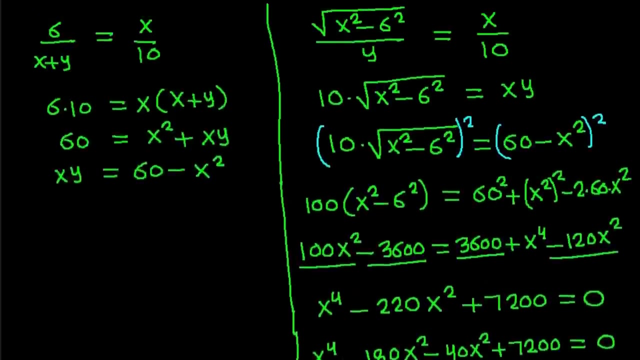 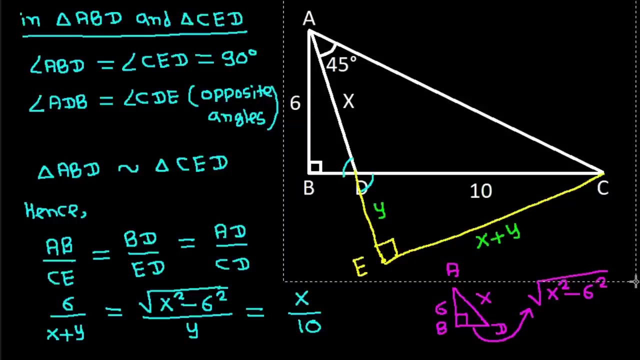 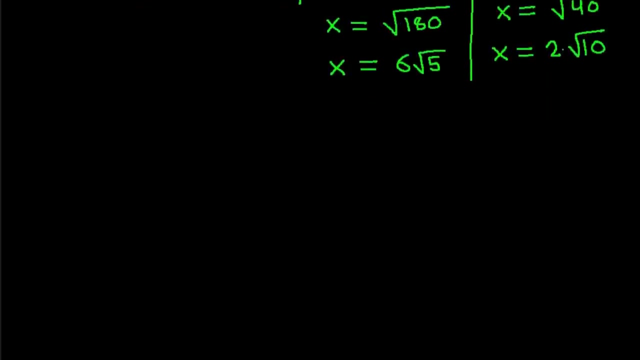 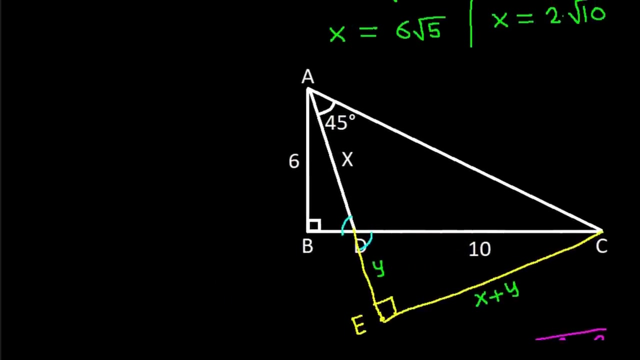 40 and x will be equal to a square root of 40. So we get: x is 2 times a square root of 10. and now inter angle: ADC. it is ADC. this angle. it is greater than 90 degree. This angle it. 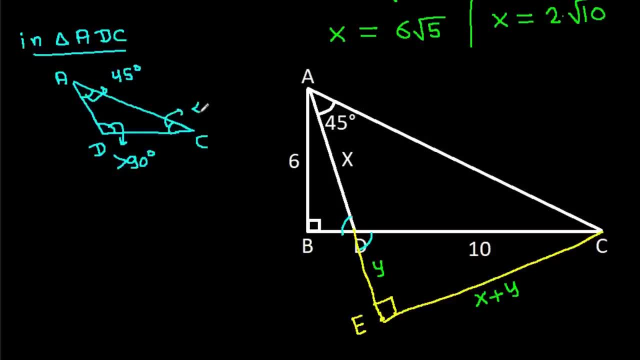 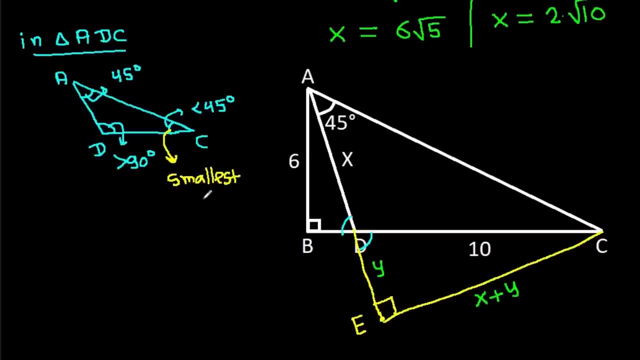 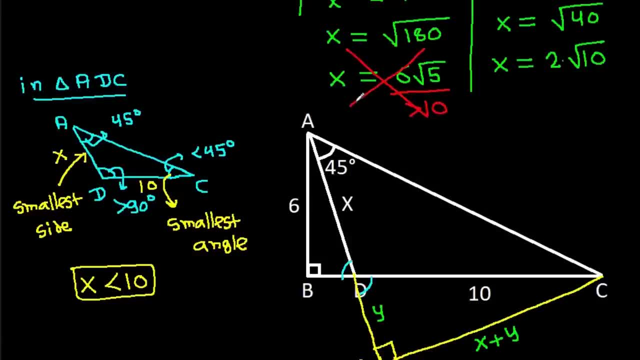 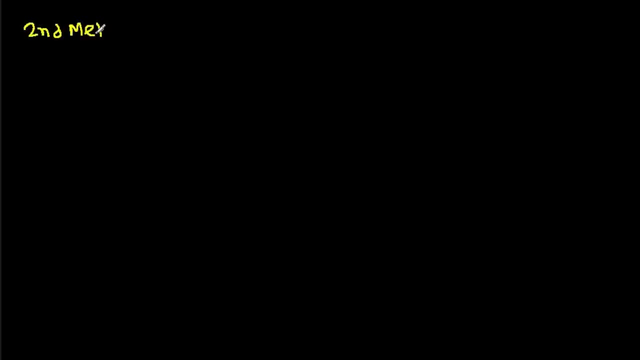 It is greater than 10, so it is not possible. That means x will be equal to 2 times a square root of 10.. And the second method: if we draw DE such that this angle is 45 degree angle, DEA is: 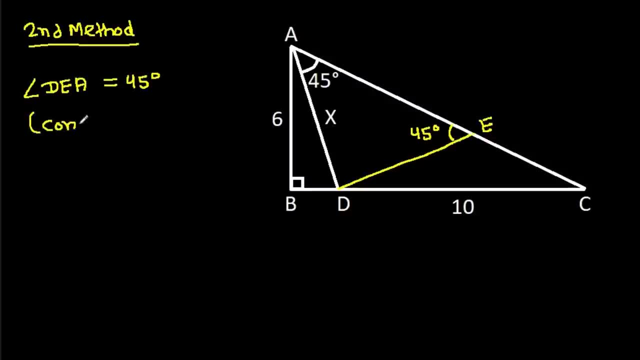 45 degree. it is our construction, then inter-angle ADE it is ADE. these two angles are 45 degree. That means AD it will be equal to DE And AD is x. so DE it will be x, DE it will be x. 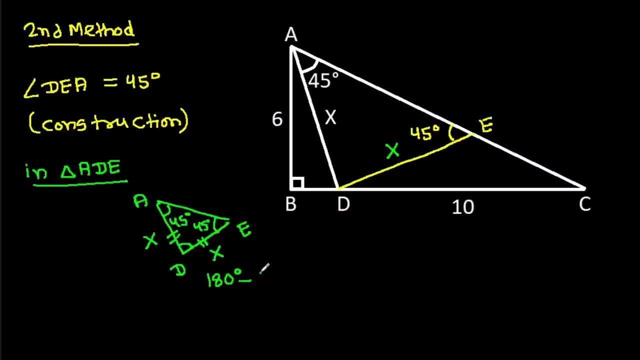 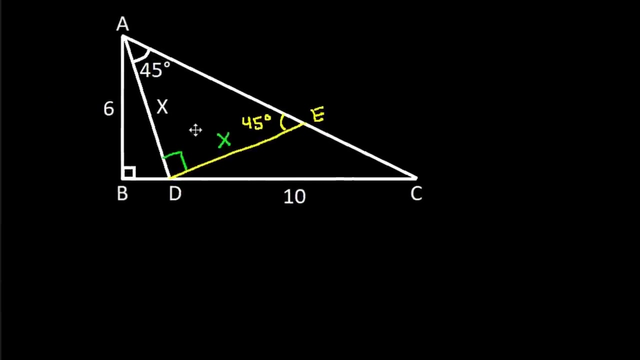 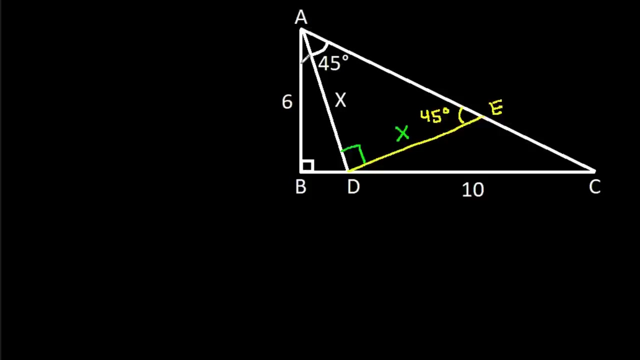 And this angle, it will be 180 degree minus 45 degree. minus 45 degree, That will be 90 degree. So this angle, it will be 90 degree. And now if this angle is theta, then this angle, it will be 90 degree minus theta. 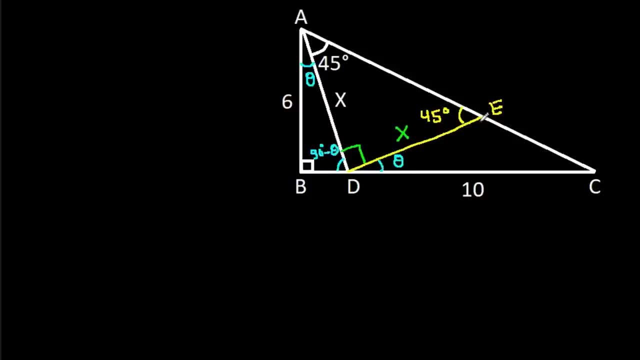 So this angle it will be theta. Okay, Thank you. point E: if we draw a perpendicular on BC- suppose this point is F- we have CD is 10 and now in triangle ABD and triangle DFE we have angle ABD is equal to angle DFE. that 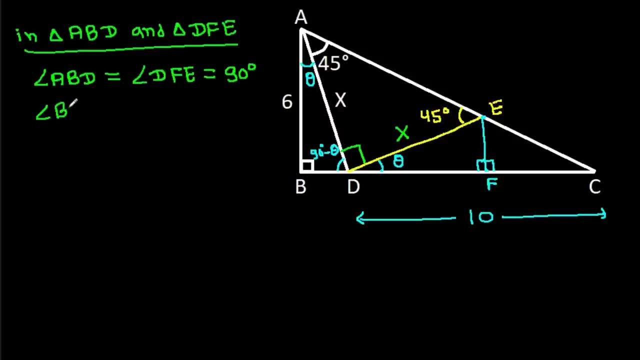 is 90 degree and angle BAD is equal to angle ABD. FDE, that is theta, and AD it is equal to DE, that is x. So triangle ABD it will be congruent to triangle DFE. Hence AB it will be equal to angle DFE. 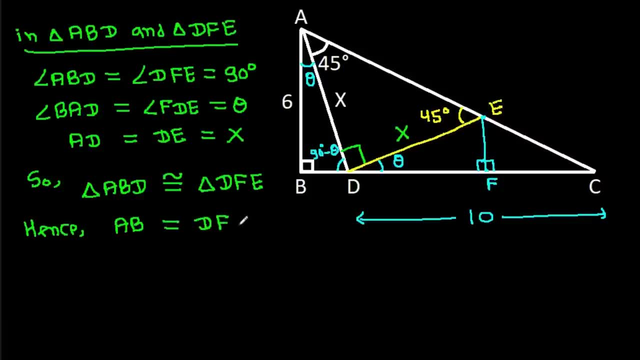 Hence AB, it will be congruent to angle DFE Hence AB. it will be equal to angle DF and AB is 6. so DF it will be 6 and FC it will be DC minus DF, that will be 10 minus 6 and it will be 4. so FC it is 4 and also BD is. 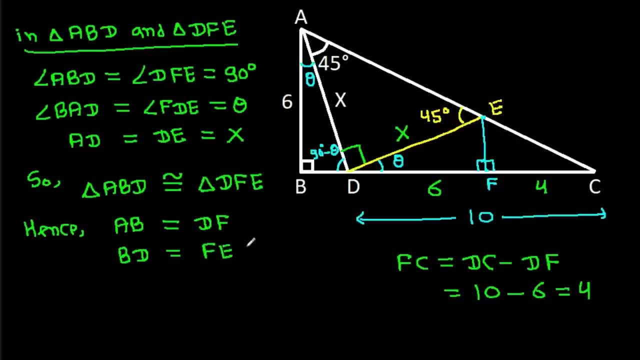 6, and so BD is 4 and it will be 4 plus 5 into 5 plus 5 plus 5 and it will be 7.. enser Now again, F has angle ABD and angle BC. it will be equal to FE. 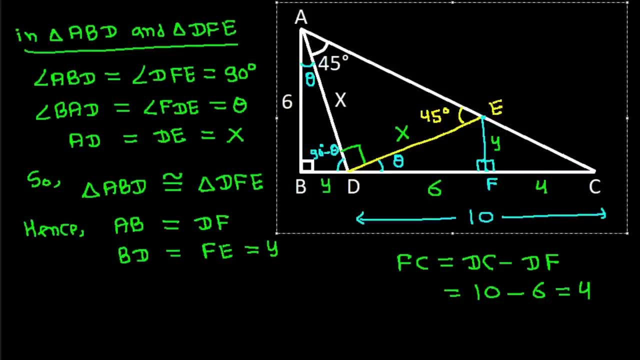 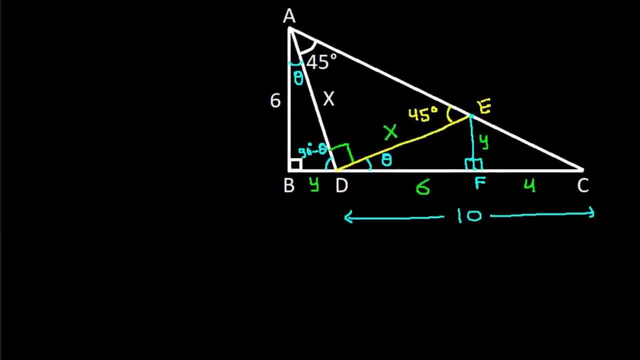 Since Y is 5, it will be equal to FE, Suppose Y. So mango Le, inside triangle, BD is Y and FE is Y and F essentially equals M. Now interangle ABC, N, E are S and they are equal. and EFC we have angle ABC is equal to angle EFC and angle ACB is equal to angle ECF. So 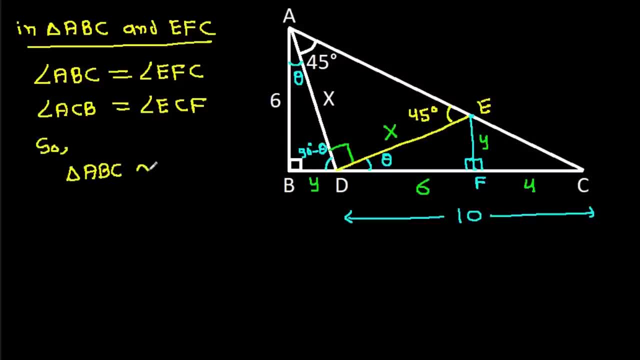 triangle ABC, it will be similar to triangle EFC. Hence AB by BC, it will be equal to EF by FC, and AB is 6 by BC, it will be 10 plus Y, It is equal to EF is Y by FC is 4 and if we cross multiply. 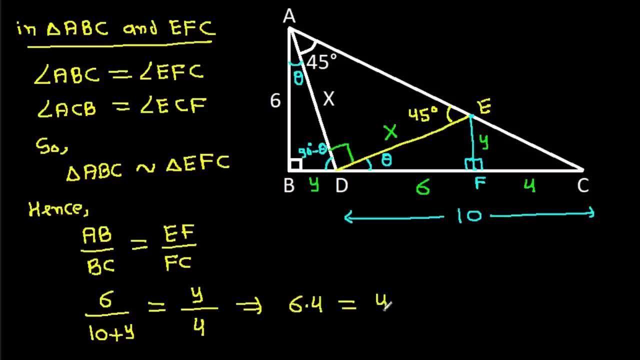 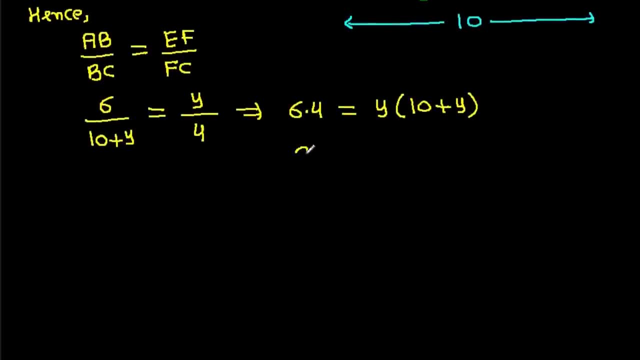 then 6 times 4, it will be Y times 10 plus Y and 24, it is 10y plus y square, and y square plus 10y minus 24, it is 0, and it is y square. 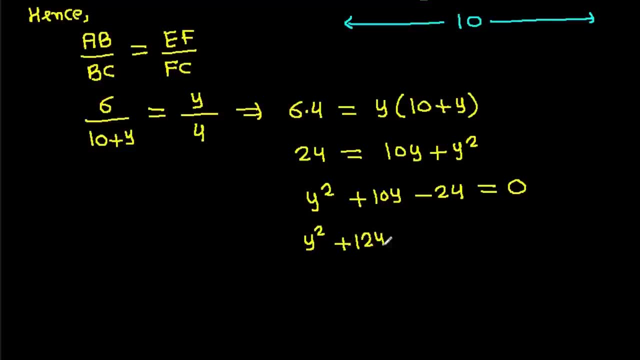 and plus 10y, it is plus 12y minus 2y minus 24, is 0.. And here we can take y common, and it will be y plus 12.. And here we can take minus 2 common, and it will be y plus 12,, that is 0. 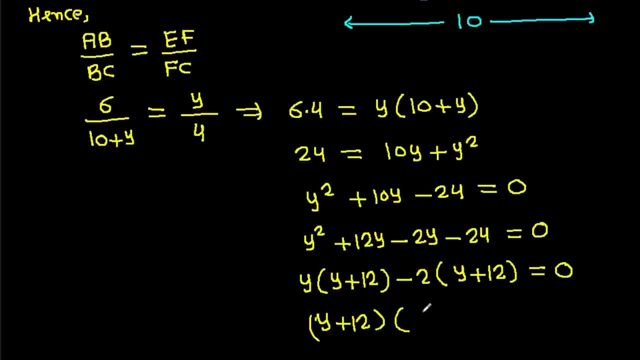 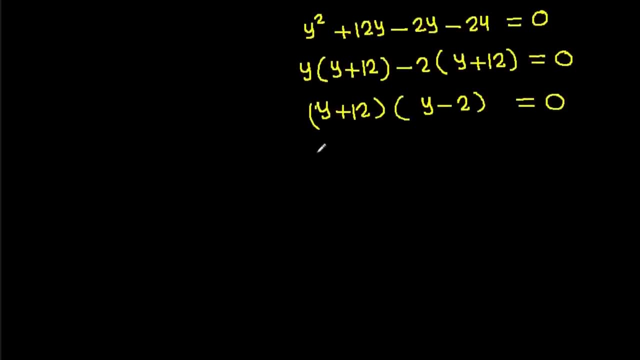 And now we can take y plus 12 common, and it will be y minus 2, that is 0.. So either y plus 12, it can be 0. That means y will be minus 12.. And either y minus 2, it can be 0. 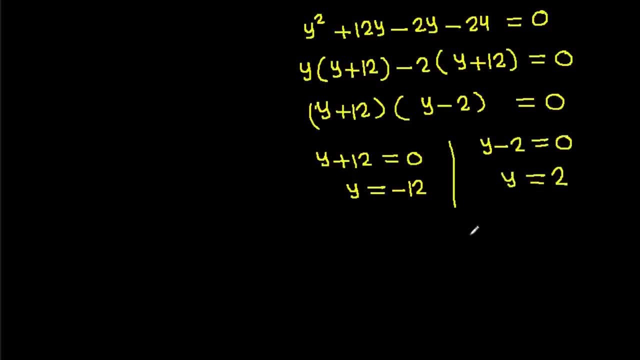 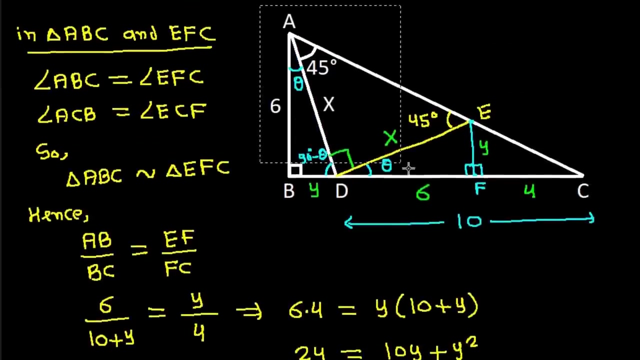 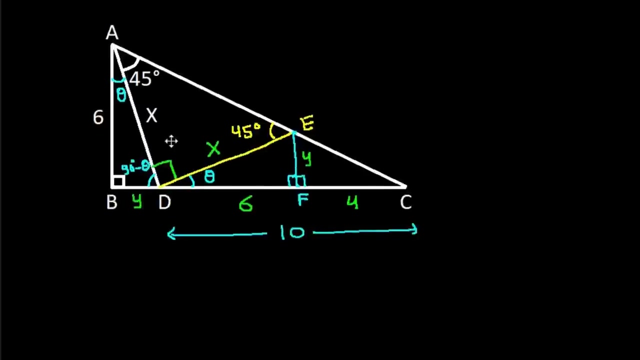 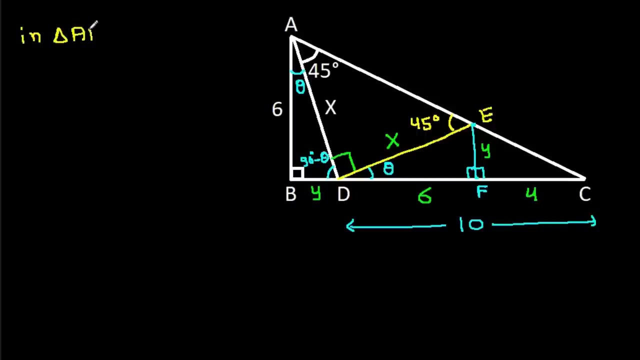 So y will be equal to 2.. And we know that y is length. that should be positive, So y cannot be negative. That means y will be equal to 2.. Okay, And now inter angle: ABD- it is ABD, AB is 6,, BD is y, that is 2, and BD is y, that is. 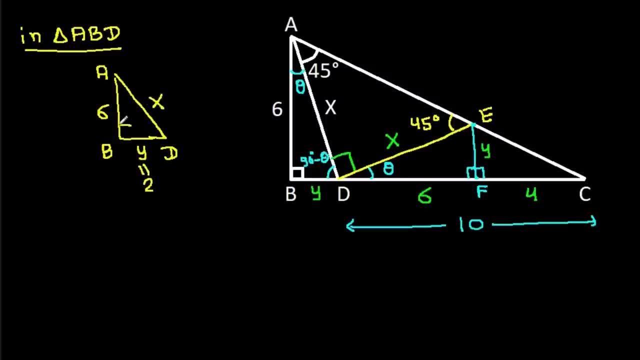 2. And AD is x And this angle is 90 degree, So x square it will be 6 square plus 2 square by Pythagoras theorem. So x square it is 36 plus 4, that is 40.. 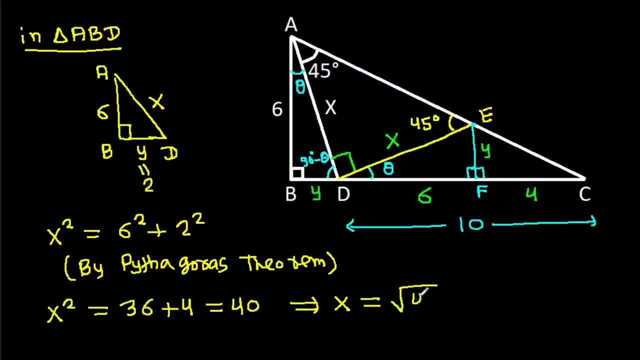 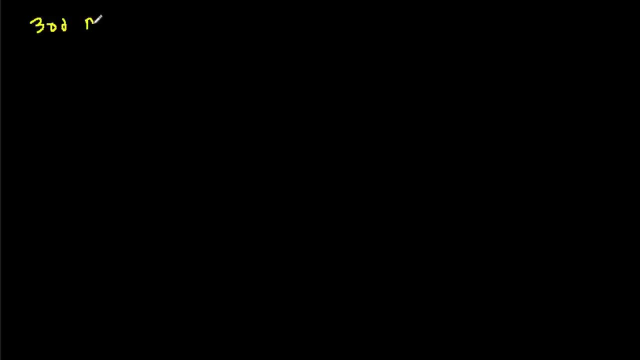 So x will be equal to A square root of 40, that will be 2 times a square root of 10.. And the third method: suppose this angle is theta And BD is y, Then inter angle ABD. it is ABD. this angle is 90 degree. this angle is theta, AB is 6,. 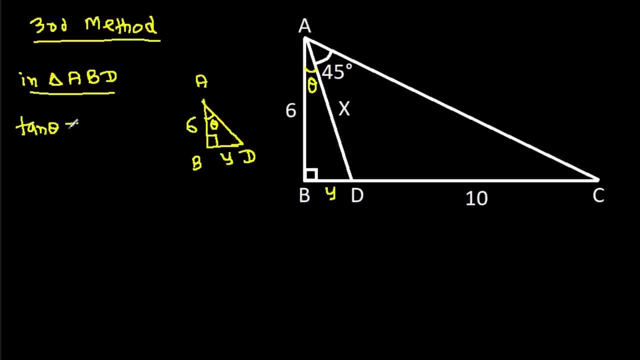 BD is y. So, tan theta, it will be BD by AB, That will be y by 6.. So, tan theta, it will be BD by AB, That will be y by 6.. So 10 plus 4 is x. 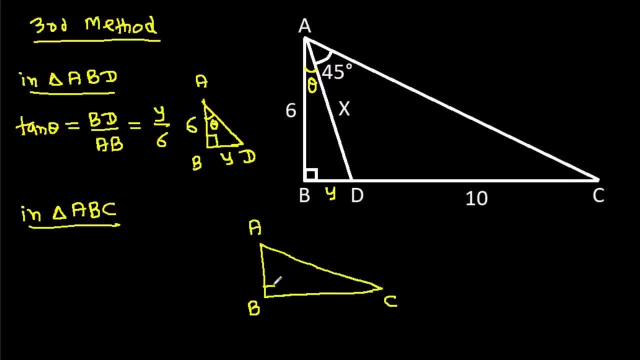 And inter angle. ABC, it is A, B, C. This angle is 90 degree. This angle it will be theta plus 45 degree. AB is 6.. BC is 10 plus y, So tan theta plus 45 degree. 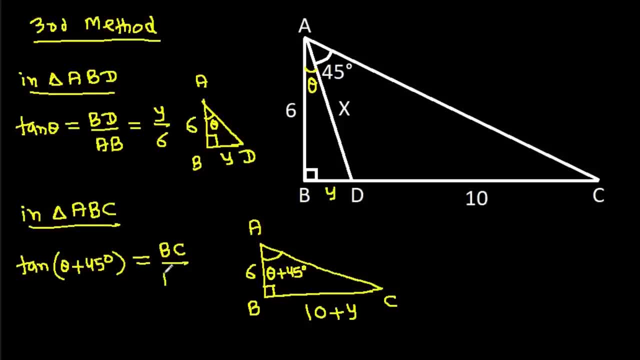 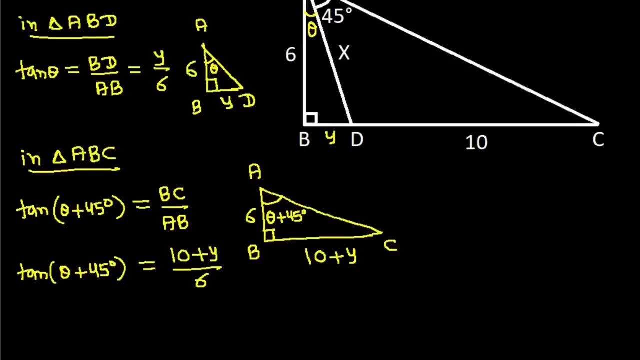 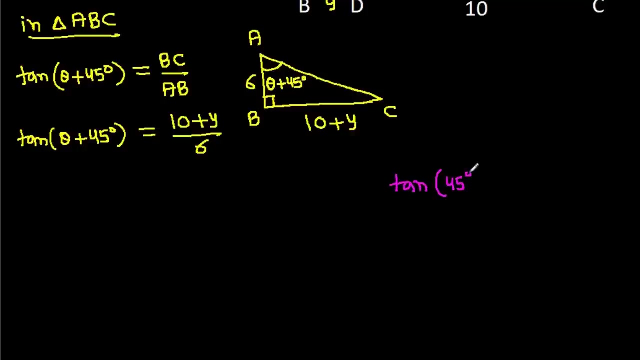 So y is 6. degree: it will be BC by AB. so tan theta plus 45 degree it is tan plus y by 6, and tan 45 degree plus theta, it is 1 plus tan theta by 1 minus tan theta, so it will be 1 plus tan theta by 1 minus tan theta. it is tan plus y by 6. 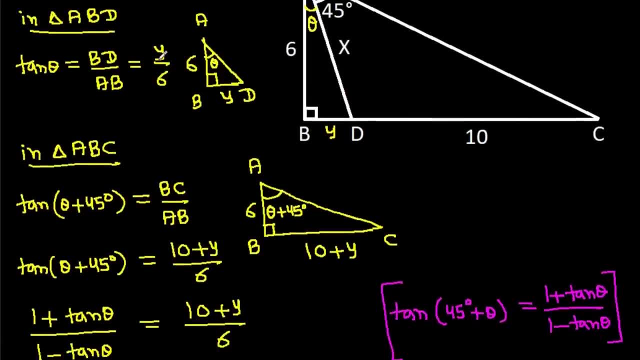 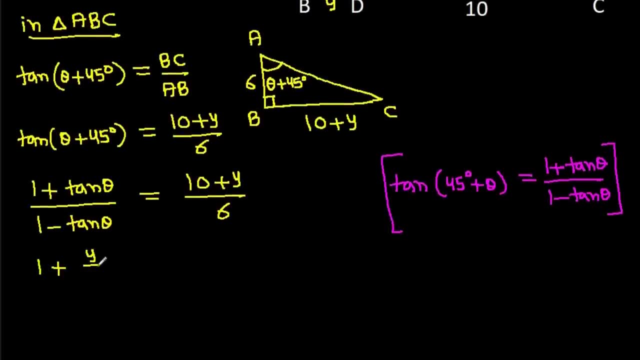 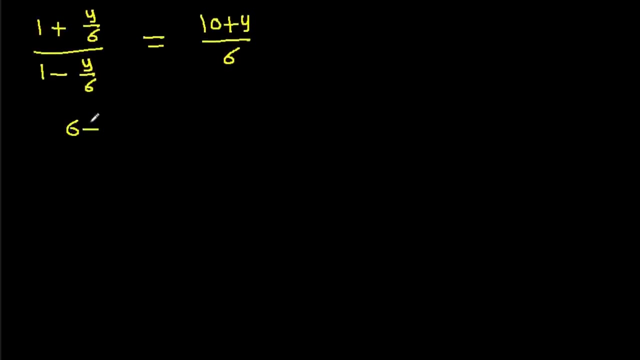 and we have tan theta is y by 6, so it is 1 plus y by 6 by 1 minus y by 6 is tan plus y by 6, and it is 6 plus y by 6 by 6 minus y by 6 is tan plus y by 6. 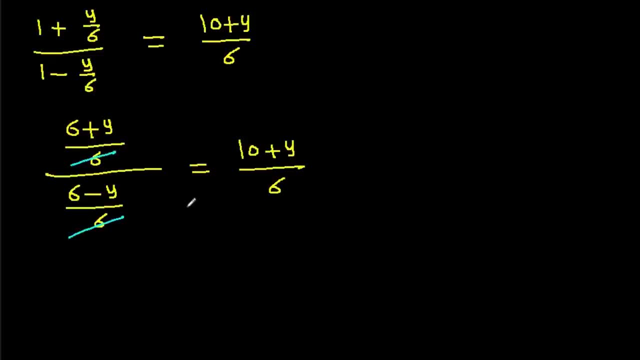 and 6 minus y by 6 is tan plus y by 6, and 6 minus y by 6 is tan plus y by 6, and 6 will get cancelled. so 6 plus y by 6 minus y, it is tan plus y by 6, and if we cross multiply. 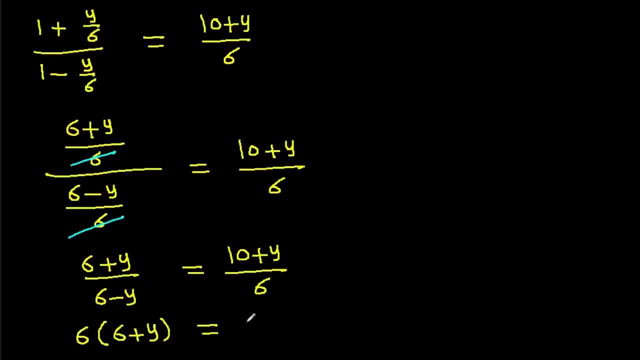 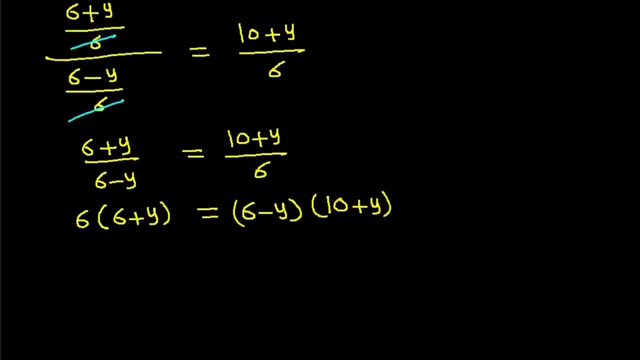 then 6 times 6 plus y, it will be 6 minus y times tan plus y, and 6 times 6 is 36 plus 6 times y is 6y. it is equal to 6 times 10, is 60 plus 6 times y is 6y and minus y times 10 is. 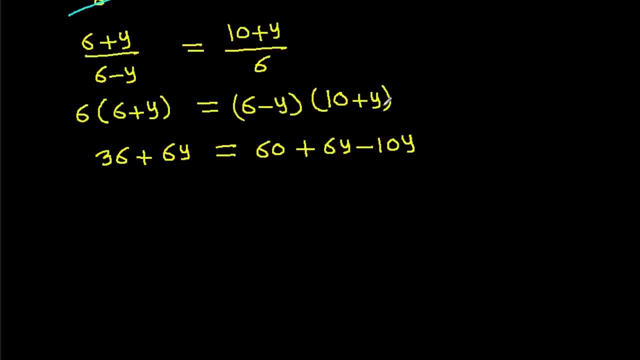 minus 10 y and minus y times y is minus y s square and 6y will get cancelled. so it is y square minus 10 y and 36 minus 60, it will be minus 24, that is 0 and it is y square. 1 is 2n y minus 2y. 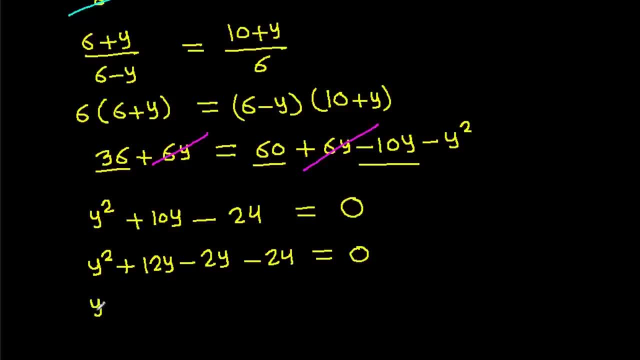 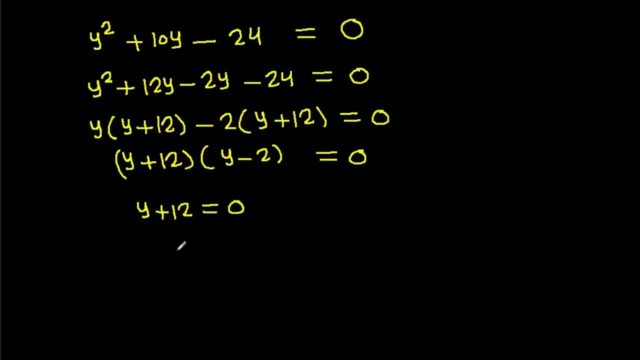 minus 24 is 0, and it is y times y plus two and minus two times y plus 2n. minus 2n minus 24 is 0, and it is y times y plus 2n minus 2n is 0, and it is y plus 2n times y minus 2 is 0.. So either y plus 2n, it can be 0.. That.